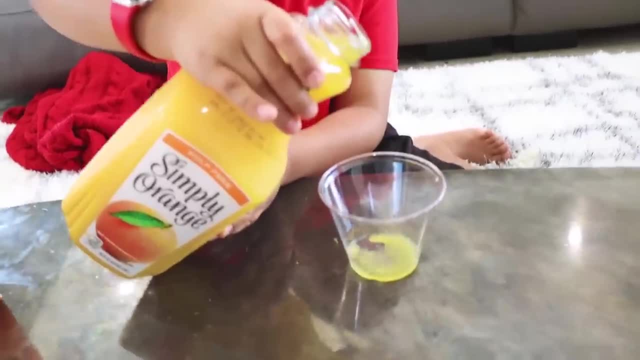 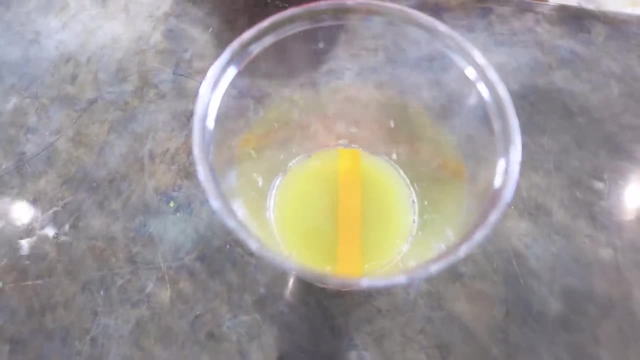 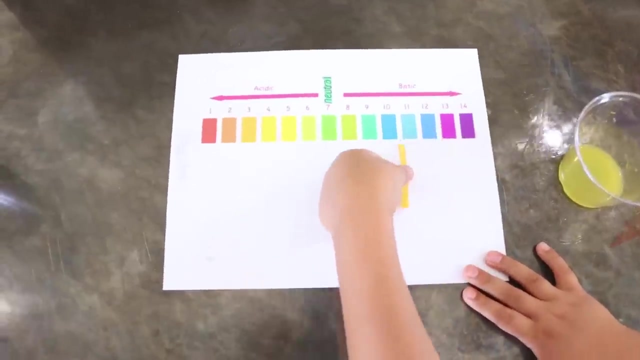 Okay, so we're going to take some of orange juice. You need a tiny bit, Is that enough? Yeah, Here is your universal indicator. Dip it in Now. we're going to take some orange juice and we're going to check it out. Ryan, I did say dip it. I wonder which one. it is All right. which one is orange? 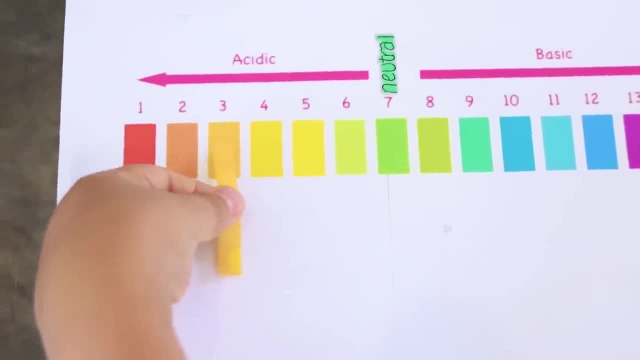 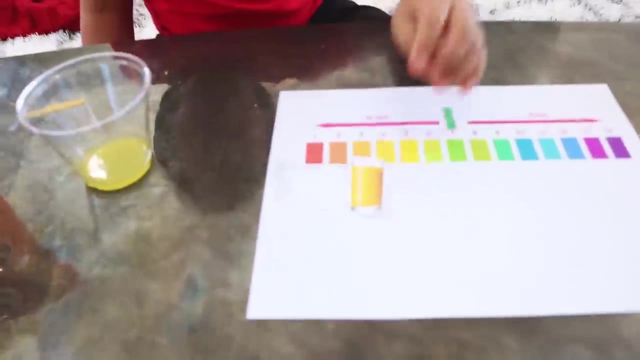 juice, Ryan. Which color is it? Oh, it's two, It's three, Three. Okay, so three is on the acidic, or basic Acidic Acidic, right here, Good job. So orange juice is right here. Yeah, so about number. 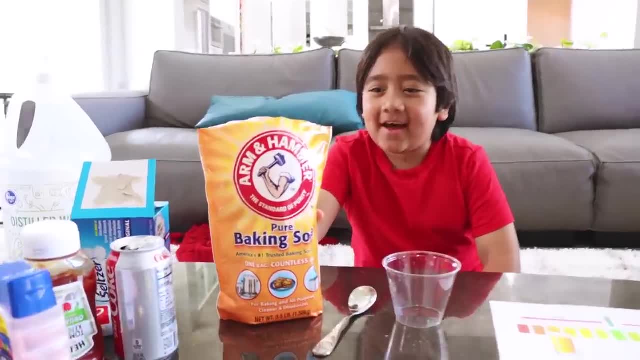 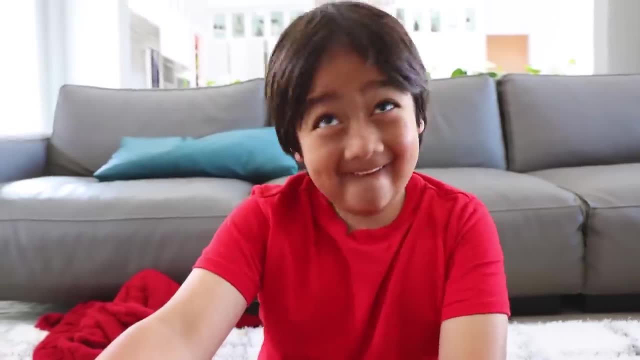 three Good. Next, I'm going to test this baking soda. All right, before you test, can you give me a guess? Acidic or basic? I feel like it's neutral. It's neutral, So Ryan thinks it's going to become. 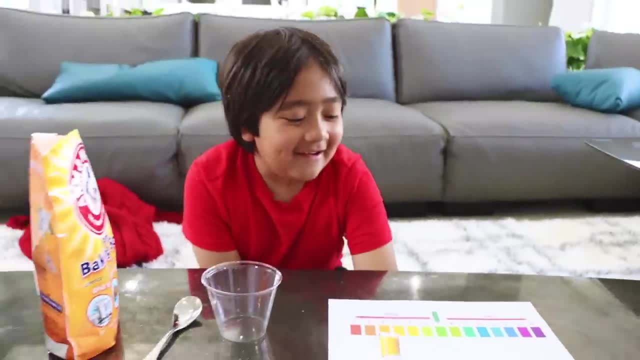 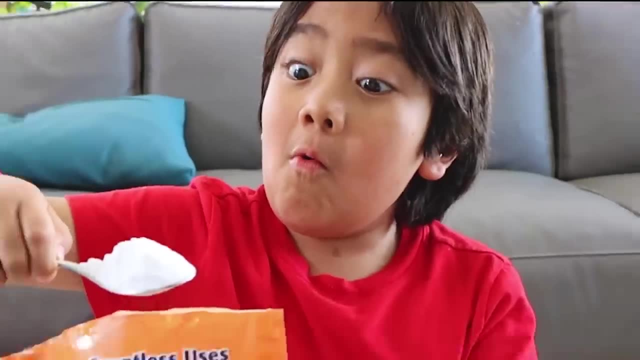 this color here for neutral. All right, let's see if Ryan is right. What do you guys think? I don't think it's acidic, but I don't think it's basic. Really Okay, let's try it. Oh, It's okay. Wow. 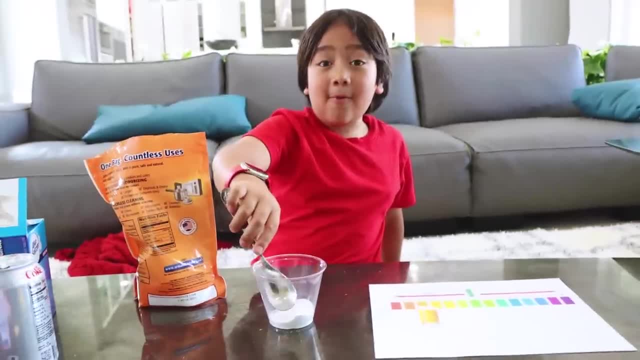 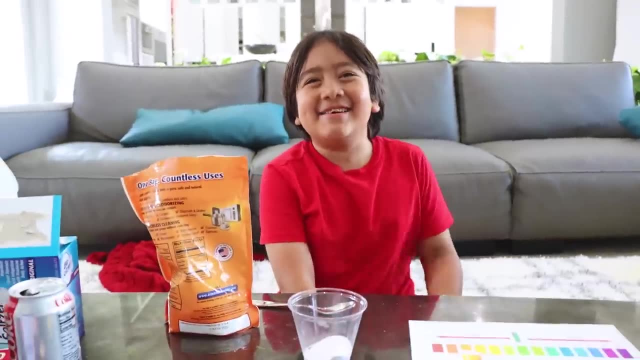 Okay. so because it's not a liquid, you know what we have to add to make it a liquid. What? Take a wild guess: Waiter, Waiter, Waiter, A waiter? Yeah, We don't have a waiter here. Water, Water. Usually pure water is neutral. 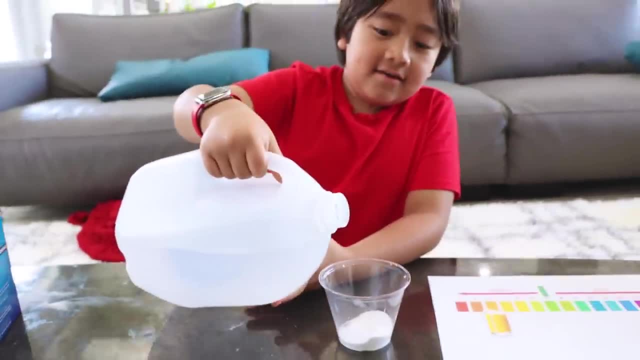 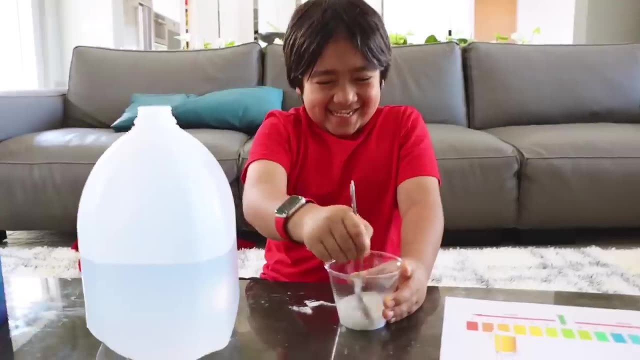 Yeah, But because a mommy had used some of these water, it's probably been exposed to the air and so it's probably a little bit acidic. but it's okay, It'll still work. I think that's good. Okay, Agitate, agitate. Don't forget to keep agitating for 10 hours. 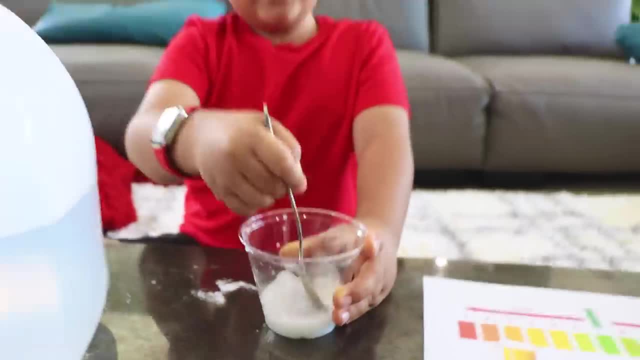 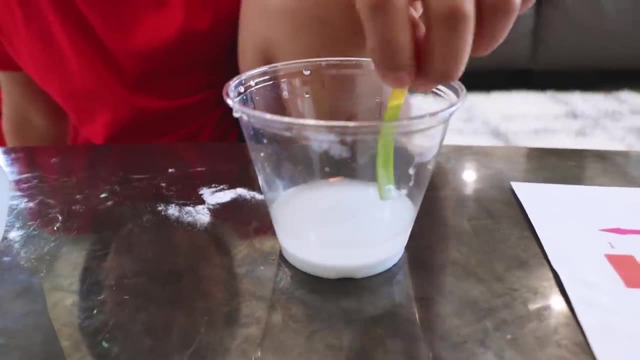 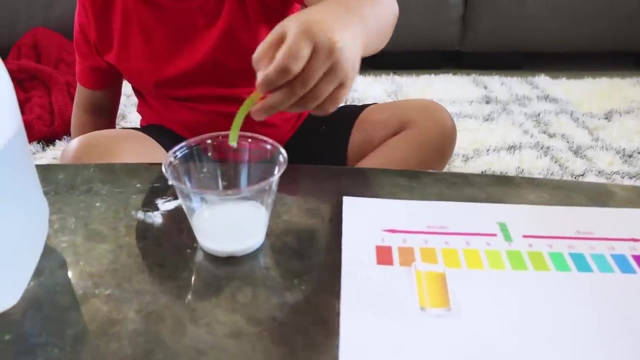 10 hours later. Just kidding, guys. Let's see if Ryan's right. Ryan is this neutral. Let's see: Wow, it's green. Okay, so let's match it up. Okay, let me dry it off. Okay, where does it go? Where does it go? 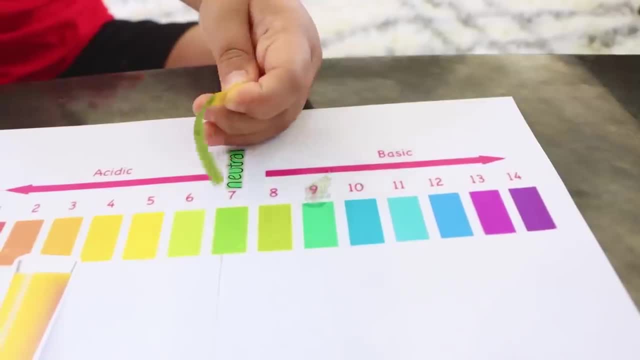 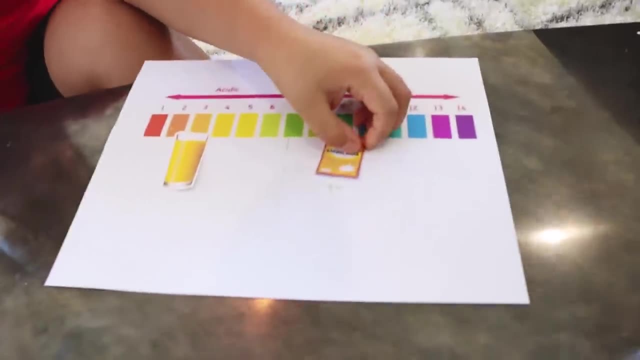 Like here. You think so. Maybe It's either basic or neutral. I'm guessing it's basic. Okay, so, basic, it is Baisique, Baisique. We got baking soda, Let's go, Let's go. 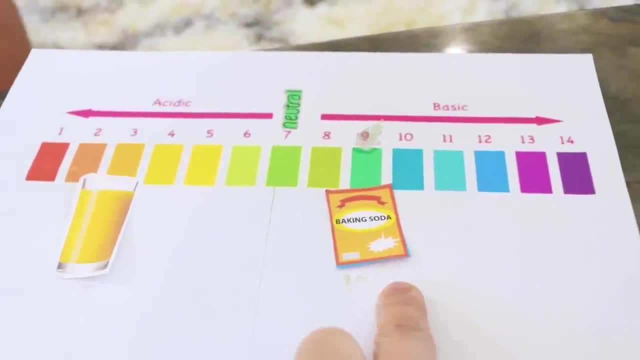 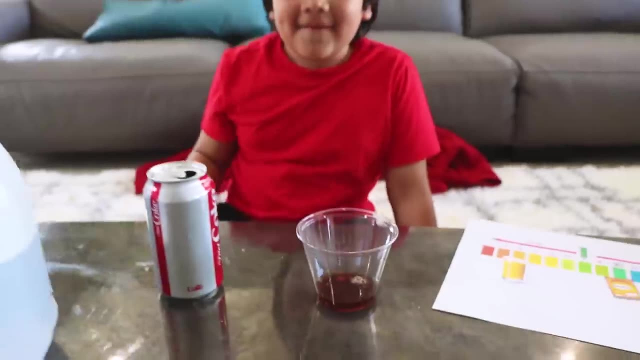 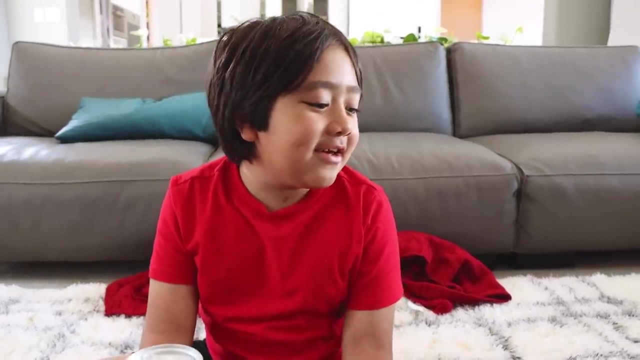 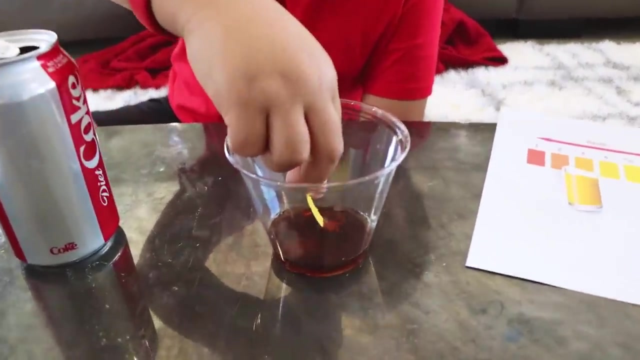 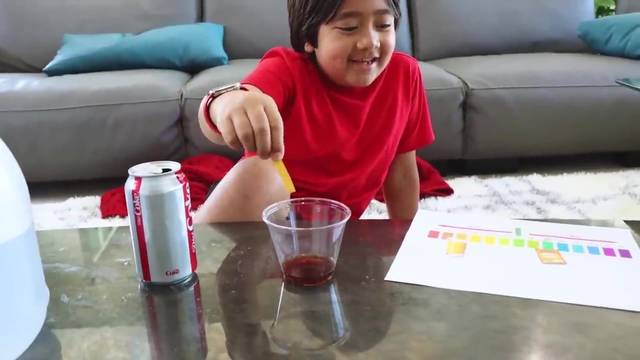 So we have one acidic so far and then one basic. next liquid I'm gonna test is soda. now, what do you guys think is soda, acid or base? my wonder, what do you think Ryan? probably a sick. okay, here's your universal indicator. let's see what indicates. it indicates in a shake. I said it, yeah. yeah, it's like the same as. 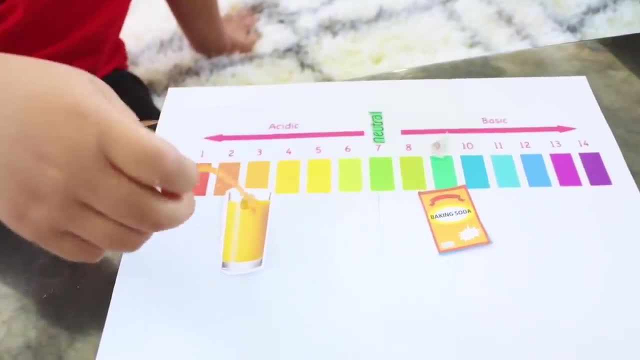 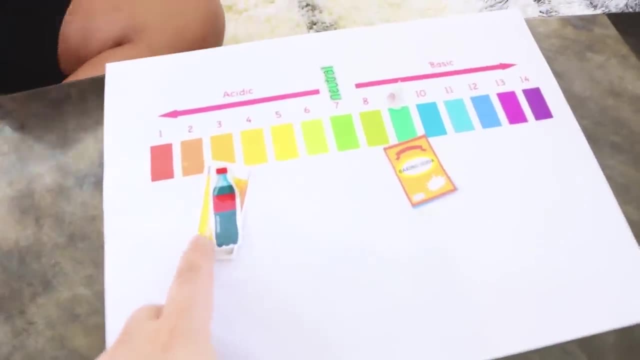 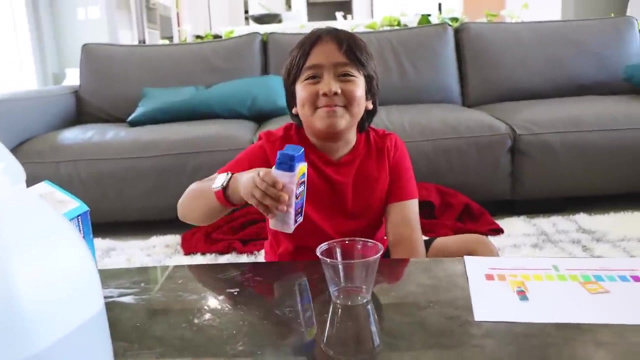 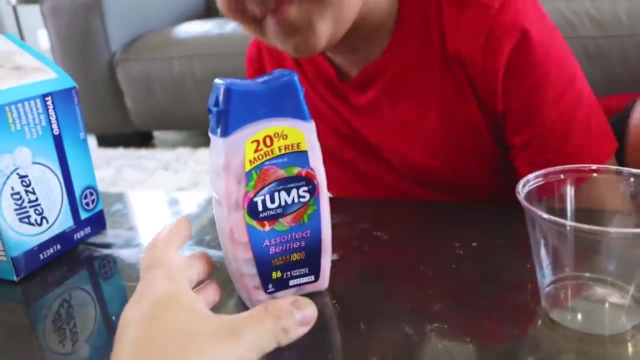 the orange same. huh, yeah, here it is on top of 11. no, not lemonade orange juice, so they're both acidic. next we're gonna try out Tom's. do you know when you use come when your tongue, that's right. when your tummy hurts, right? so let's figure out: is the Tom and? 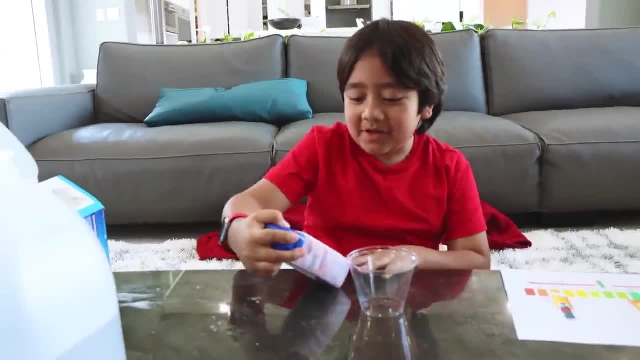 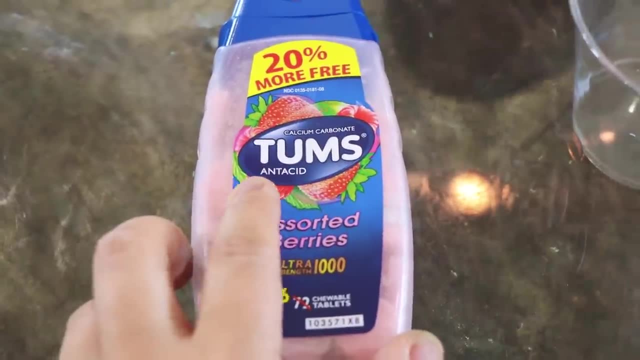 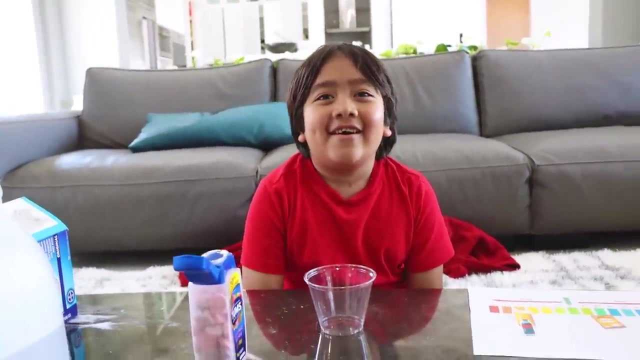 acidic or basic? what do you think acidic? okay, look at the name of Tom's Ryan. it says a Tom's is in an acid. what is? and think about the word. and like anti, bullying, antisocial. what does that mean? it means again, again, so, again, acid. so 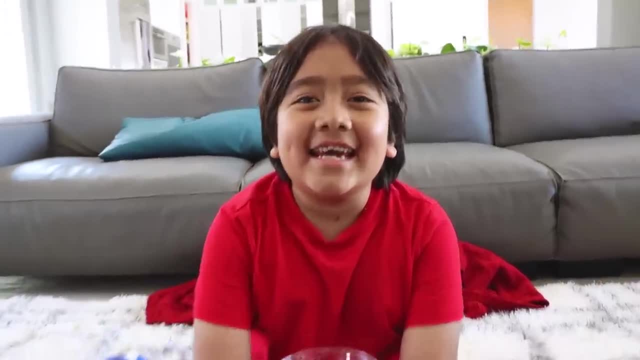 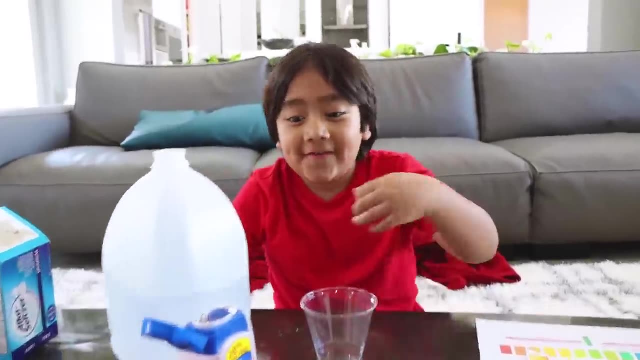 what's the opposite of an acid? and antisocial. what does that mean? it means again again, so, again acid. so what's the opposite of an acid? and basic, basic, but we'll see if it's right. okay, so first, because this is not liquid, you're gonna have to put it in, you have to put in water, water, get. 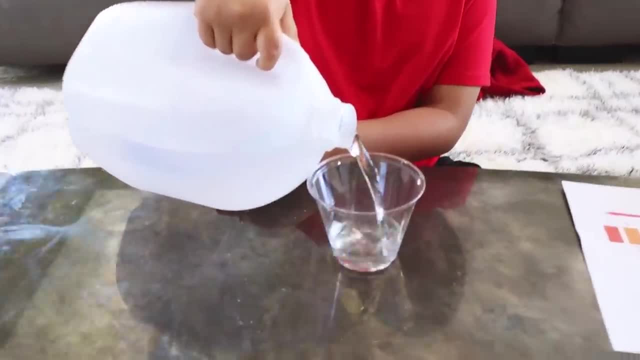 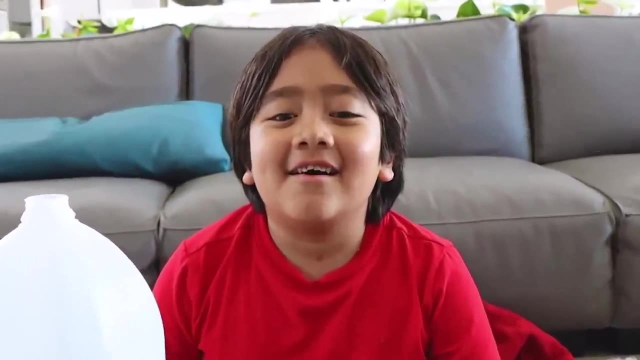 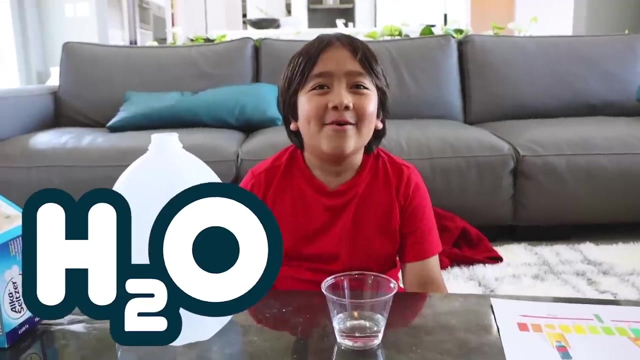 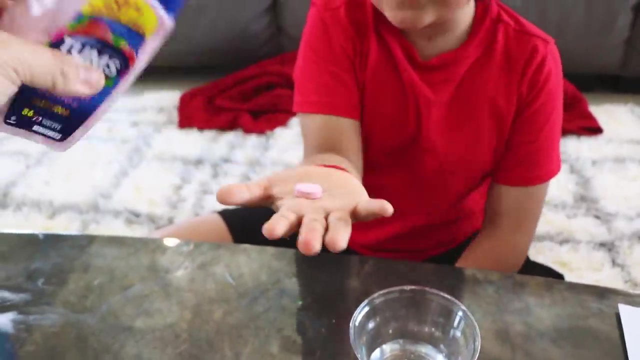 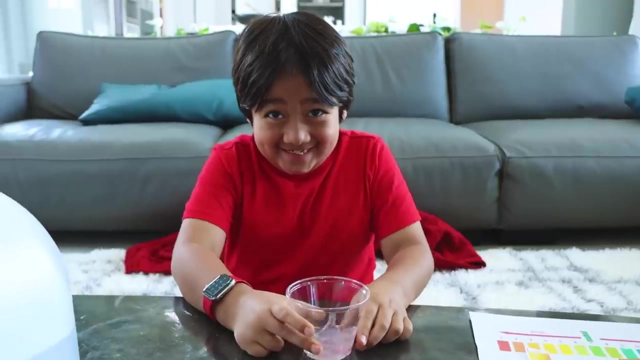 Brian's pouring some water. Ryan bonus question for water. do you know the chemical compound of water, what? what is the symbol of our kids of water? h2o? h2o comes for you, it comes. have fun, shake, shake, shake that we might have to crush the time. 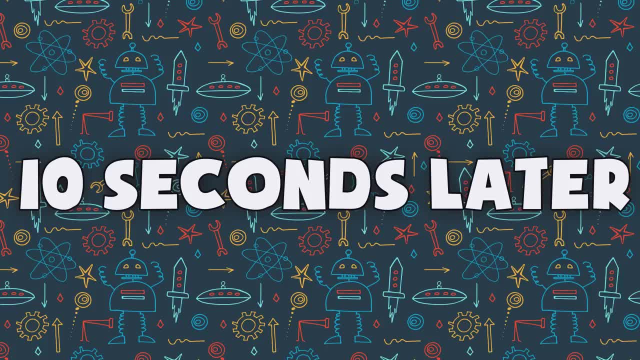 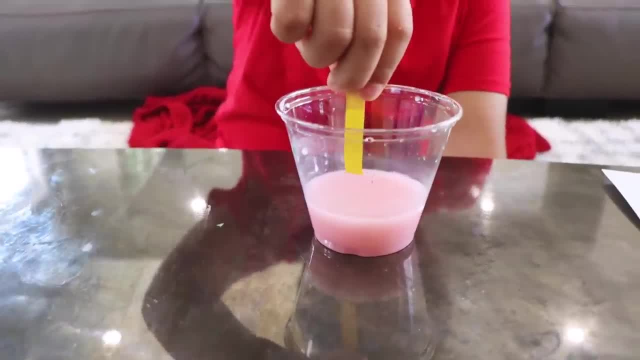 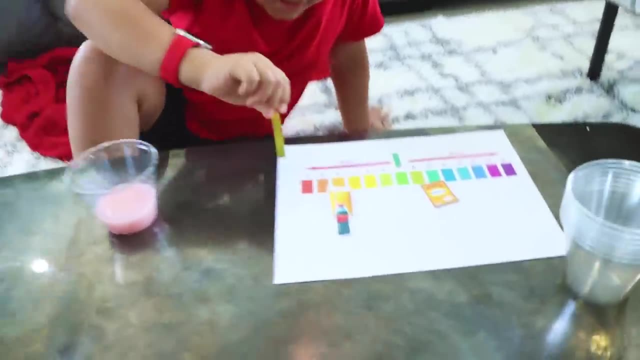 10 seconds later. now we put in the universal indicator and it says it's an eight. okay, so let's test it out against the chart. Okay, let's see. so it's none of these. I think it's this one right here, It's eight. 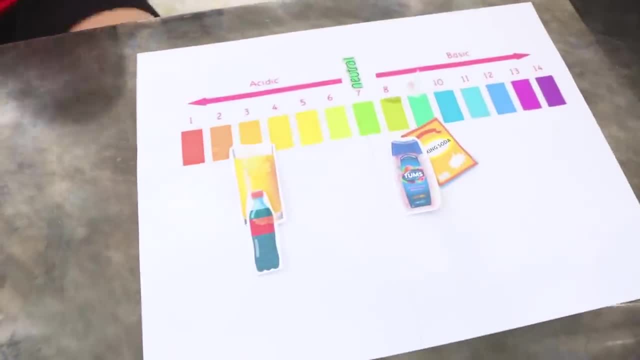 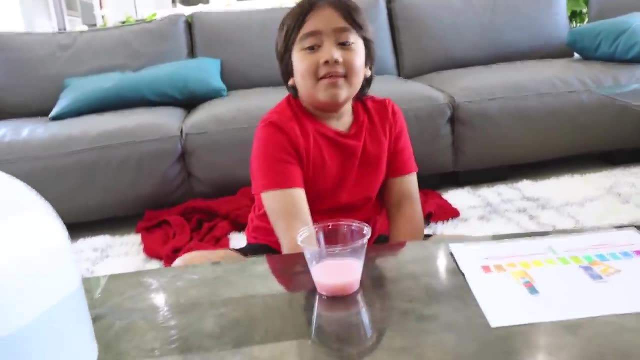 Yeah, Yeah, looks good. Okay, here we go. Tums is a basic, That's right, yeah, So when you have a tummy ache, it means your tummy is maybe too acidic, so you want something to fight against the acid. 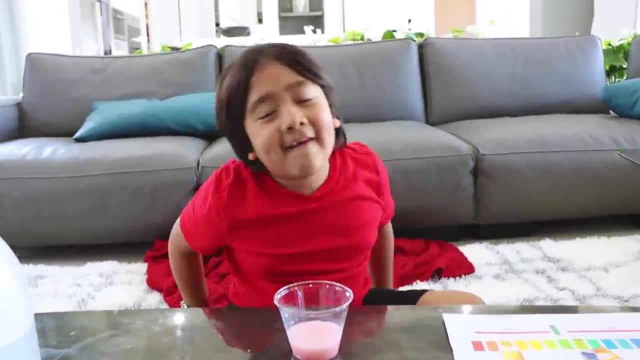 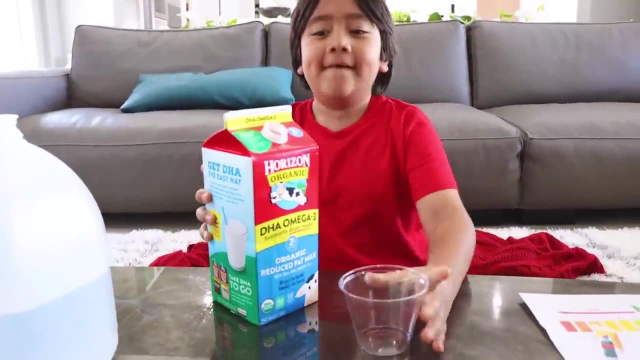 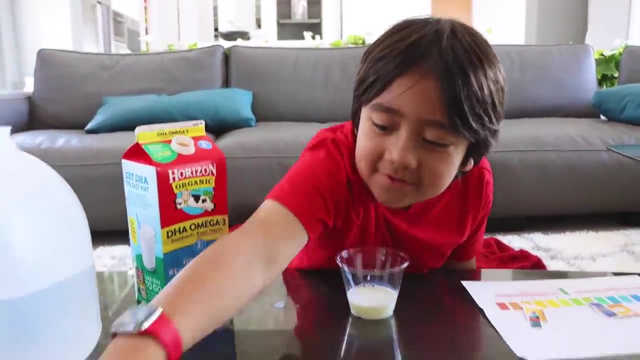 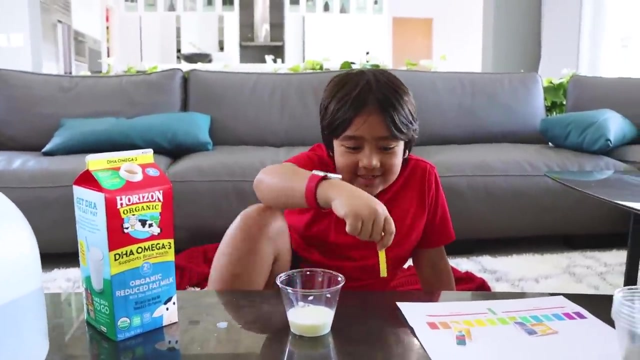 which is something basic, To neutralize it. yeah, Now we're gonna try some milk, my favorite drink in the world. Okay, Good, Oh, And now the universal indicator. What is it indicating? It's indicating this one, I think. 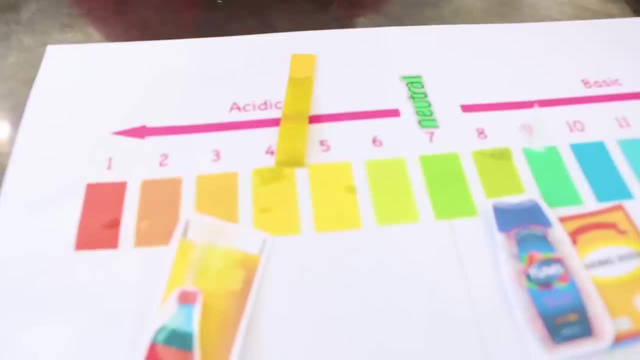 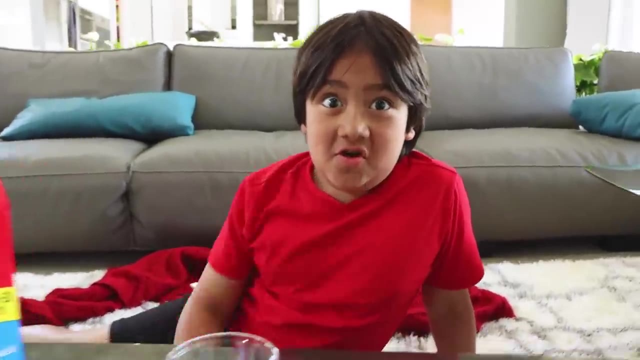 Five or four. they kind of look exactly the same. Oh, Kind of between a four and a five, right, Yeah, Okay. so what does that mean for milk? It means it's a drink. It's acidic, Okay, Acidic. 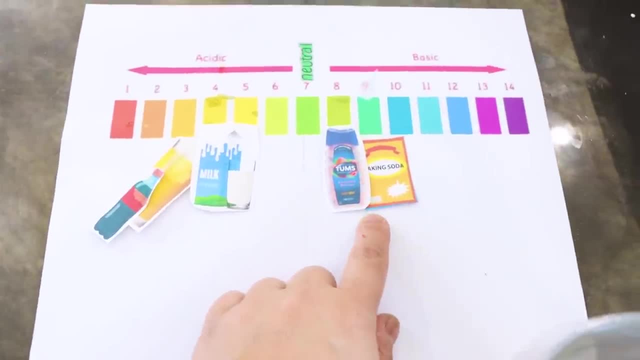 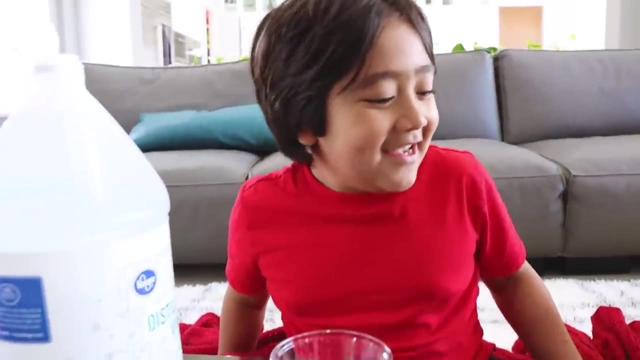 So far, these three things are acidic and these two things are basic. Next we're gonna try out vinegar: Shh shh. I think it's acidic, You think so. I think it's number one or two, You think it's that strong? 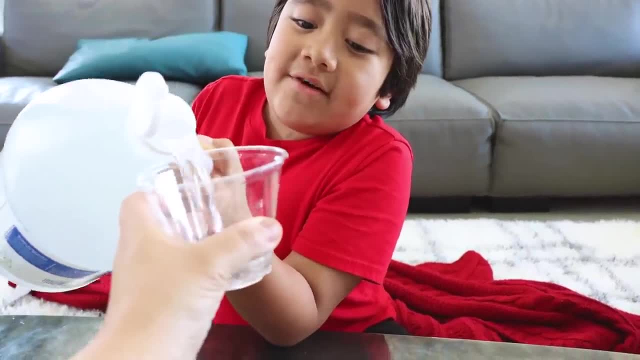 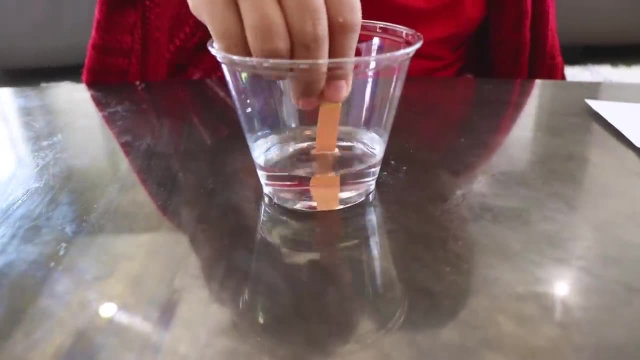 Yeah, Okay, let's see. Ooh, oi, oi, oi. That's enough. there you go. That's enough. Now I'm gonna use a universal indicator. Wait, it's number two. Yeah, it's number two. 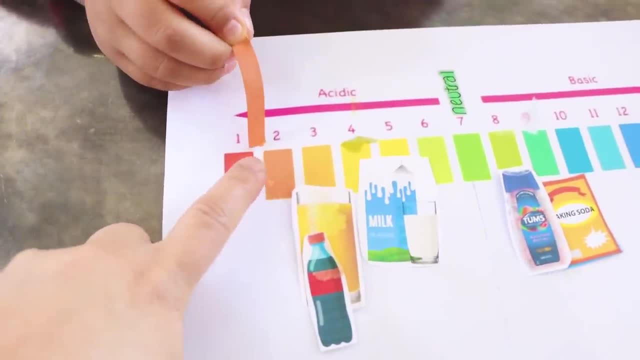 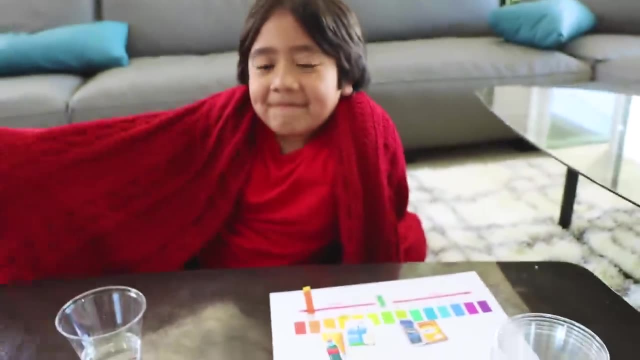 You're right, Ryan. yeah, So what does that mean? Is it more acidic or less acidic than the milk? Um, more acidic, That's right, more acidic. So here is neutral. neutral is seven, So the further you go away from neutral. 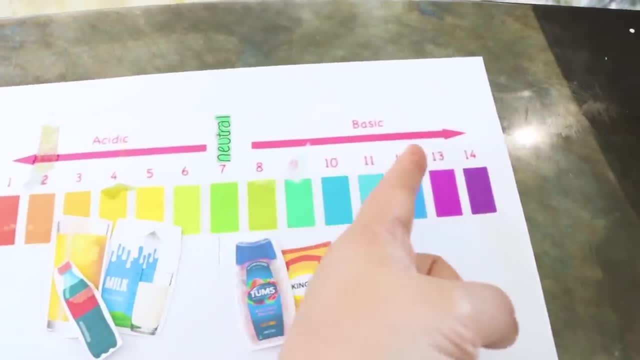 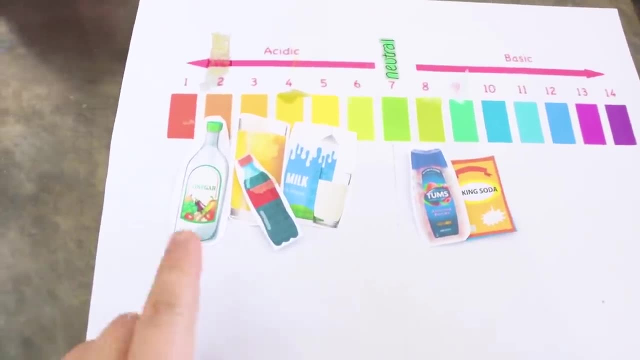 this way, the more acidic it is, And then the further you go away from neutral this way, the more basic it is. Vinegar goes right here. There you go. So which one of these are the most acidic Vinegar? Vinegar, because it's further away from seven. 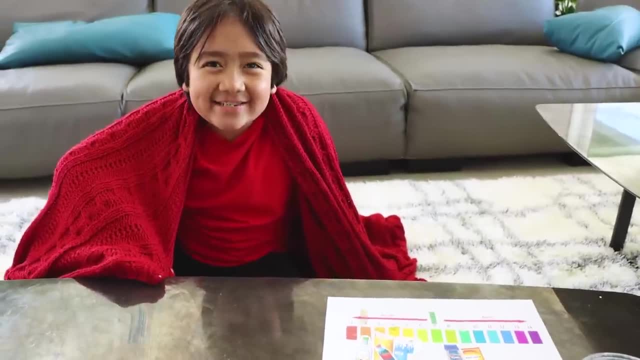 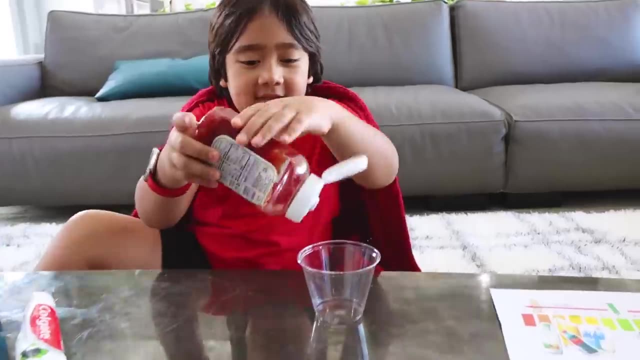 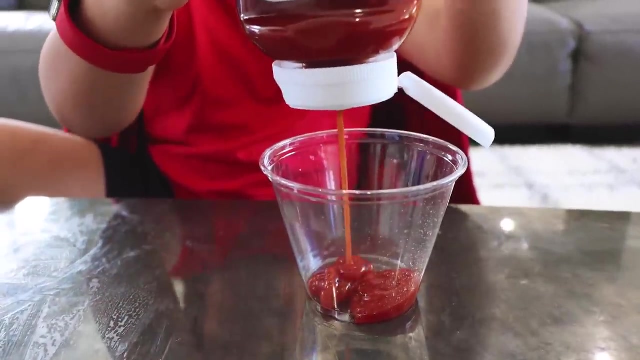 Good job. The one that is the most basic is basic soda. Basic soda, Yeah, Baking soda. Next, I'm gonna test out ketchup, Ketchup, Ketchup. There you go, Perfect. We have to actually put a little bit of water in. 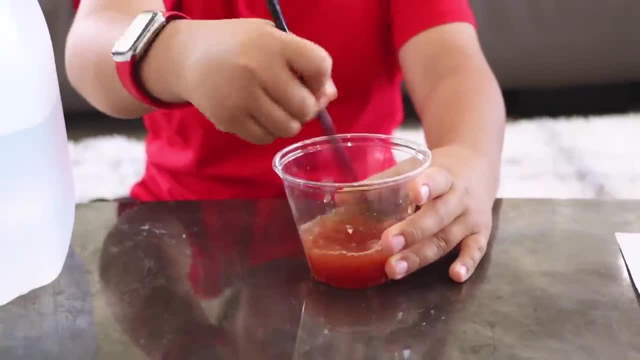 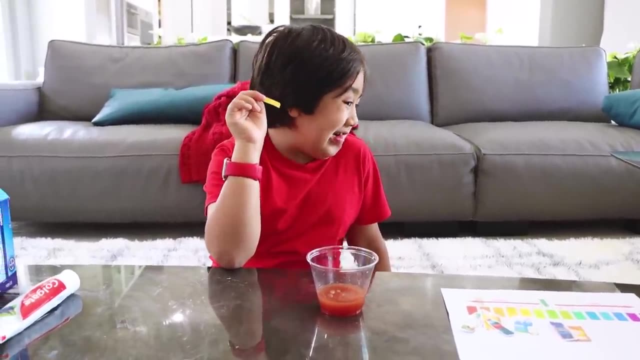 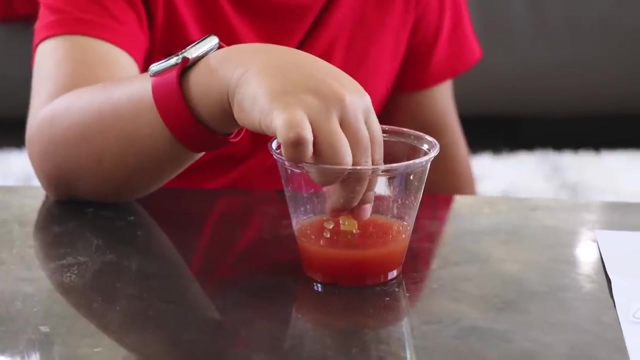 Yeah, Agitate, agitate. So what do you think it is, before you use the universal indicator? Probably Basic, Basic, okay. No, I think acidic, Acidic, Acidic, It is acidic. Okay, which number? 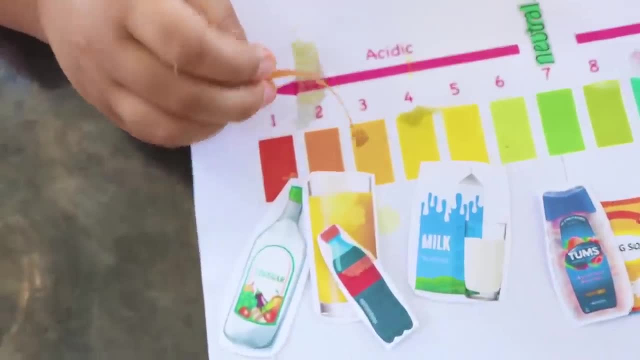 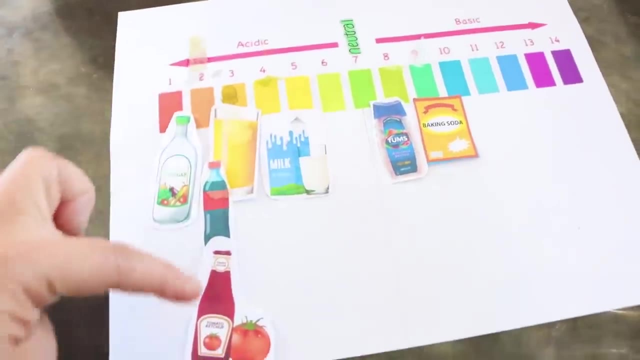 Let's see. Wait, it's number three. Another three. Yeah, Well, we have three, threes. Yeah, you guys, if you notice, you've been eating and drinking a lot of things that are acidic, correct? Yeah? 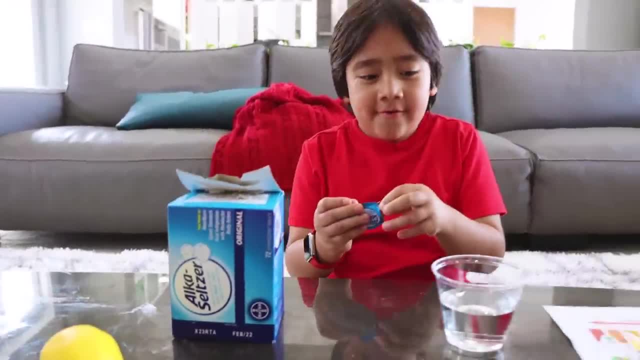 Next I'm gonna test out. Next I'm gonna test out Alka-Seltzer. Okay, do you think Alka-Seltzer is acidic or basic? Probably basic, Basic. Yeah, so you also use Alka-Seltzer. 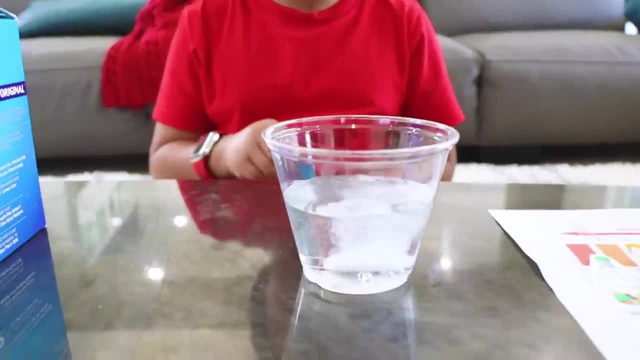 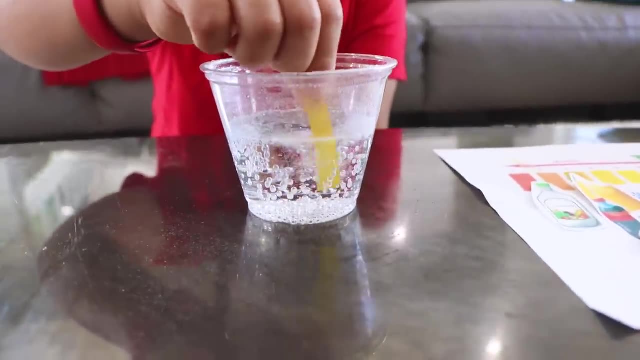 if you have like a tummy ache, So it's also an antacid, Whoa. but I like Alka-Seltzer. Look how it fizzes and bubbles. Yeah, put it in And you- Whoa, it actually didn't change color. 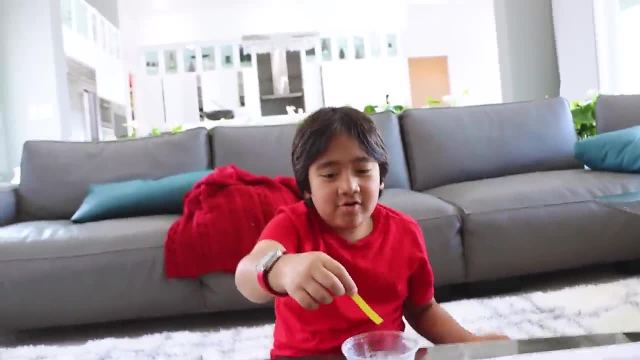 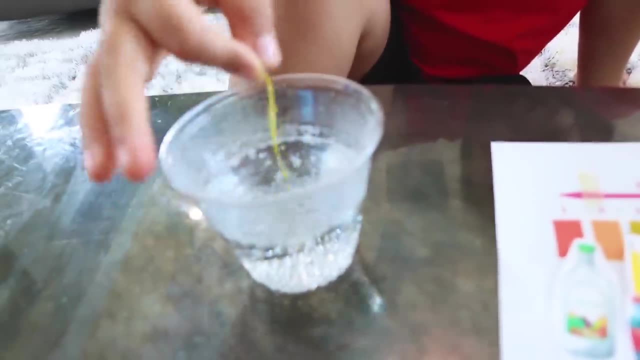 Really Interesting. Hmm, that's interesting. Oh wait, no, Let's try it. Oh, so maybe you have to wait for it to dry. Yeah, because it kind of looks green. Okay, all right, I'm gonna wait for it to dry. 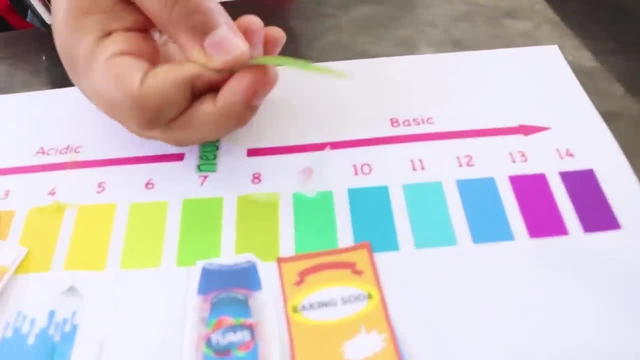 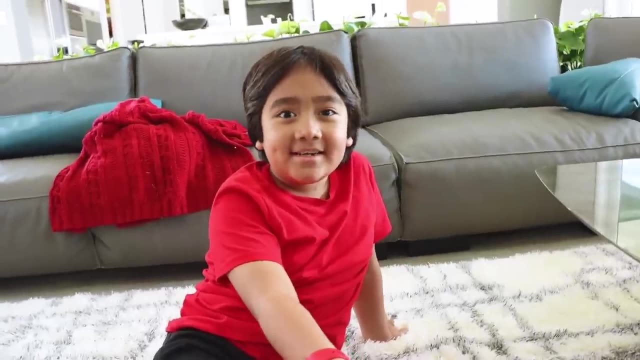 Hmm, let's see what it is. Oh, I think it's a number: nine. It's a basic. Okay, yeah, it's a nine. So is it a weak basic or is it a strong basic? It's a weak basic. 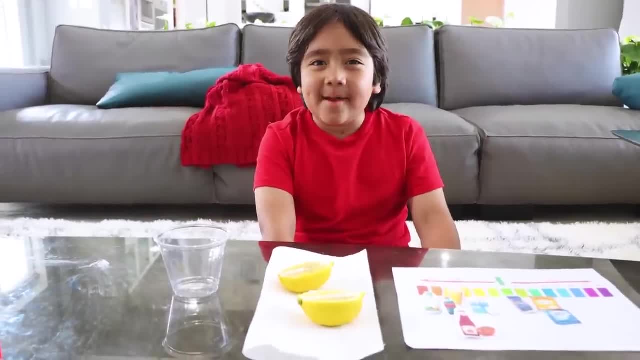 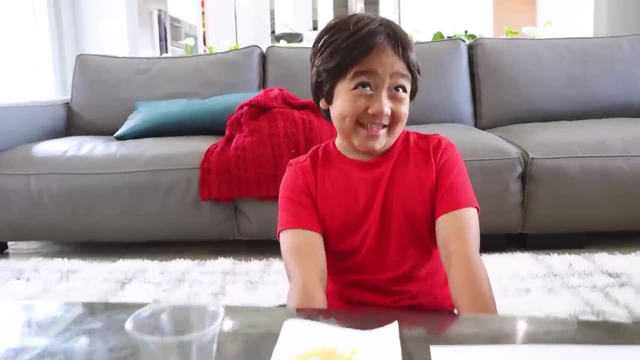 And there you go. Next, I'm testing out lemon. Do you know? lemon is really sour. So do you think lemon is acidic or basic? Probably acidic, Really Okay. Okay, It's probably gonna be a three, two or a one. 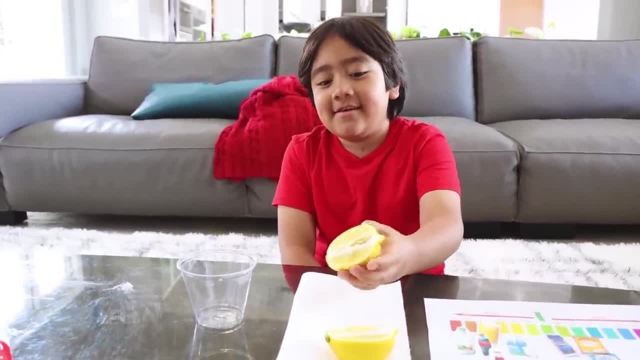 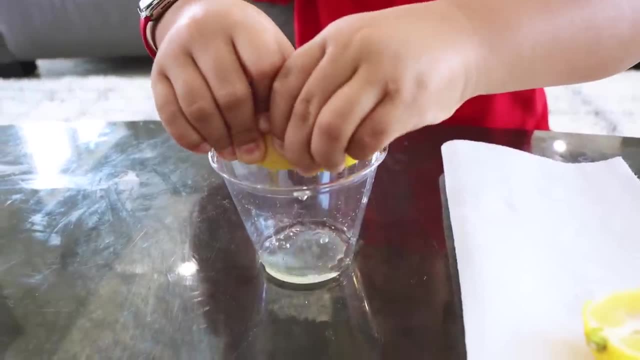 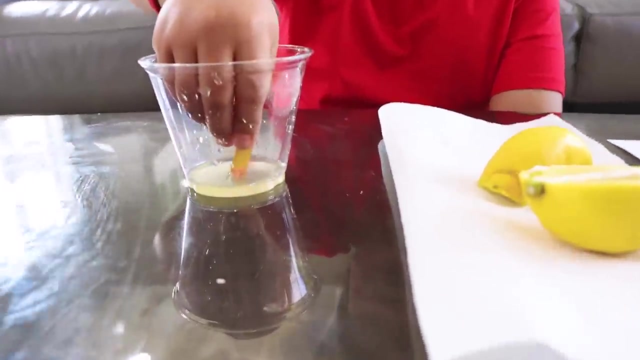 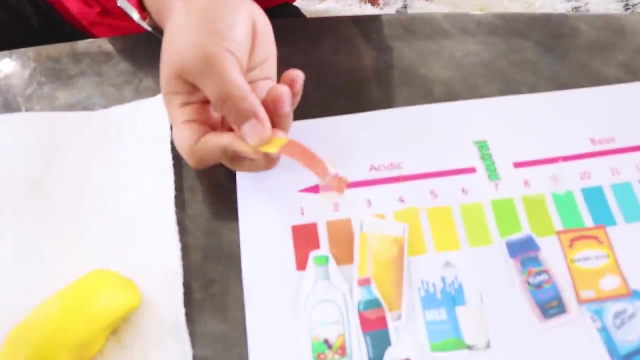 That's strong, Yeah, Okay, let's test it out. Okay, I want to use two hands. Now let's put it inside. It's probably acidic. It's number two. It's that acidic, Whoa. Oh yeah, you're right, Ryan. 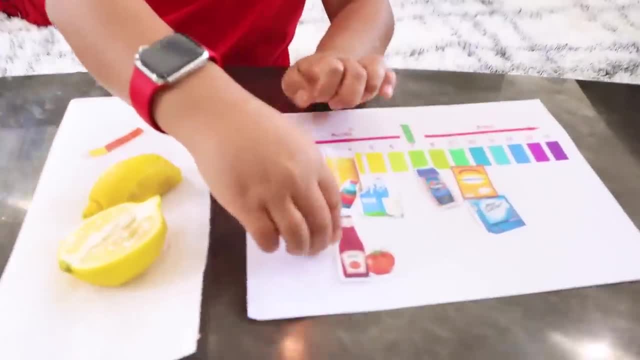 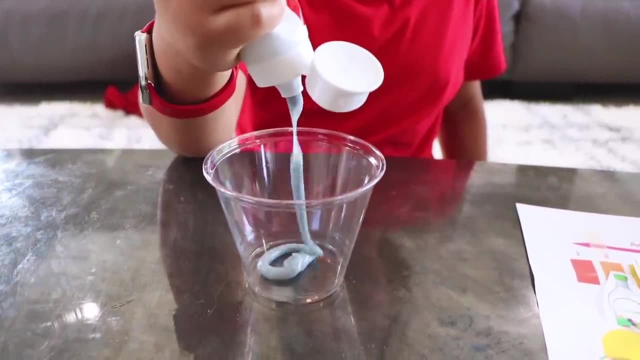 It's pretty strong. huh, Yeah, we can put it right after the vinegar. Now the last thing we're gonna try is some toothpaste. Ooh, I'm pretty sure we need to put water. That's enough Agitate. 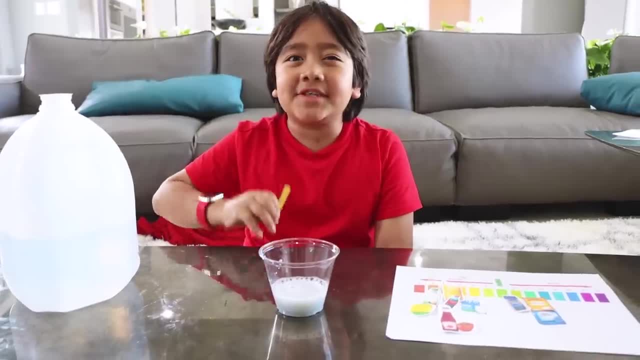 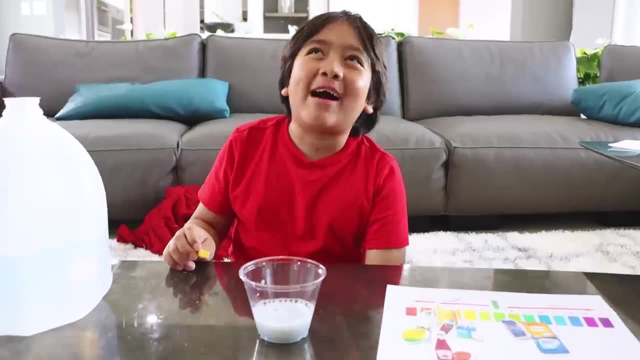 Agitate, agitate. it's probably done Time to use the universal indicator. Wait, What do you think? it is Probably neutral. Neutral I mean no, not neutral. I meant a basic, A basic. I'm gonna say it. 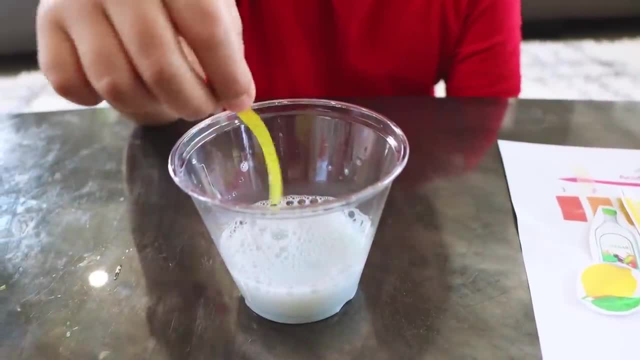 What do you guys think? Okay, you gotta wait for it to dry. Wait, I think it's already green. It's getting green, but it's still wet. so we're gonna wait for it to dry a little bit. But yeah, it's already turning green. 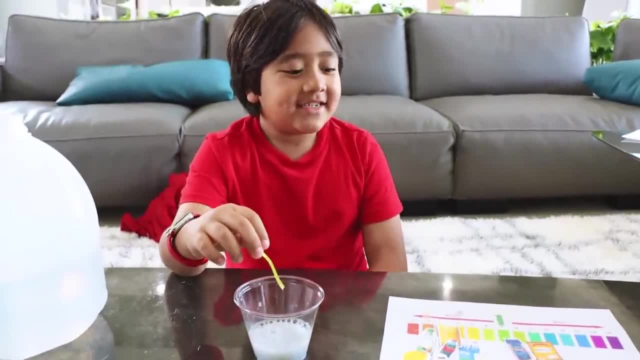 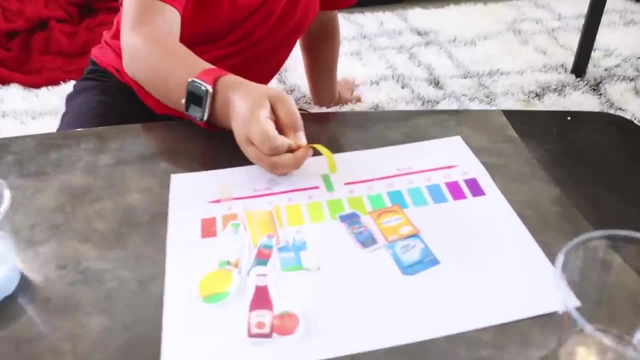 So it's either a neutral or a basic. Okay, Seven or eight. Let's wait a little bit longer, Let's see what it is. I think it's an eight. An eight, Yeah. So what does that mean? That means it's a basic. 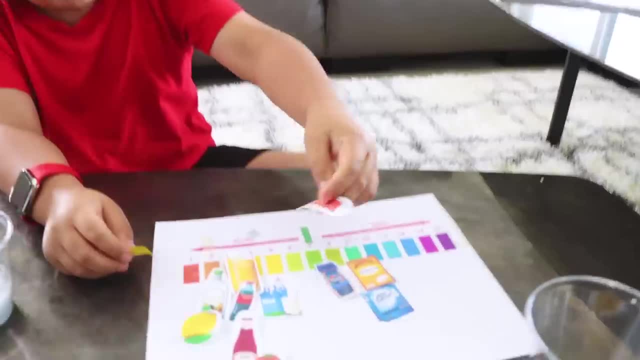 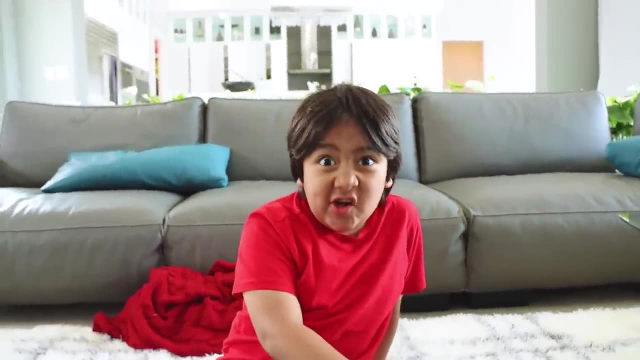 Basic. here you go, Here is your lube of toothpaste. Basic: A lot of things that you drink and eat are Acidic Acidic. So that's why Dun, dun, dun, Since a lot of the things that you eat and drink. 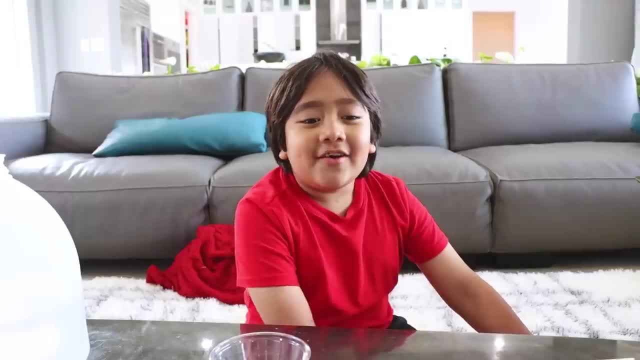 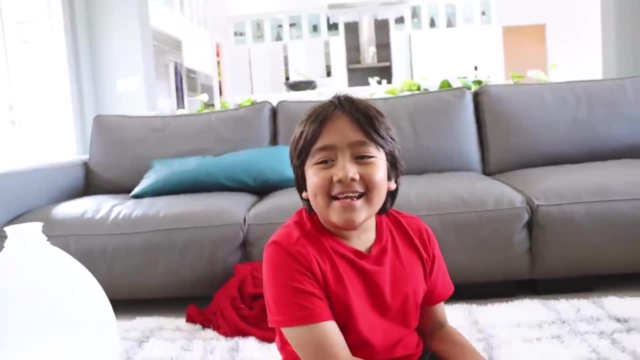 are acidic. how do you get rid of it? Like what's the best way? you think You eat and drink and put on your teeth? basic things, Basic, right. So that's why you have to use toothpaste- and toothpastes are basic- to get rid of the acid. 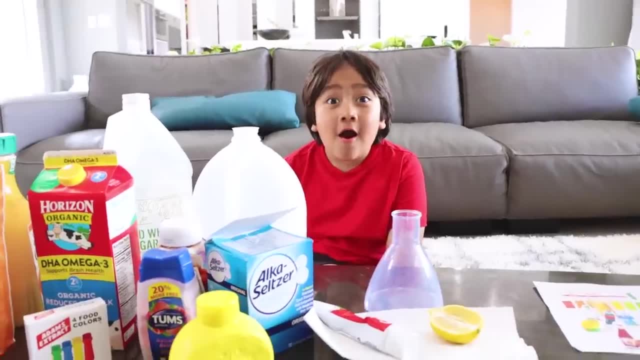 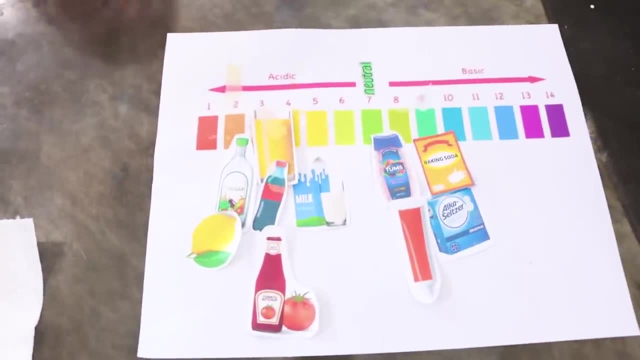 Ah, Do you know how we in the video? I want to ask you, Ryan, do you know how we always do the baking soda and science experiment video? Yeah, According to the chart, which one is an acid and which one is the basic? 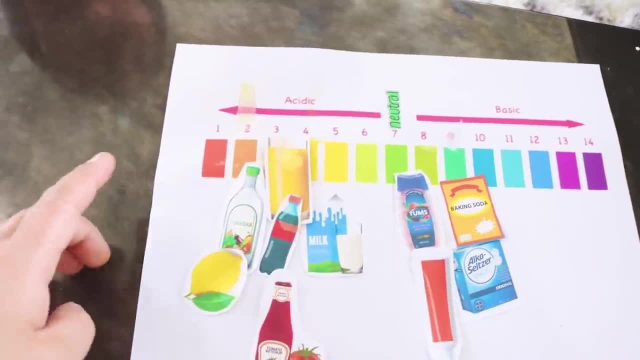 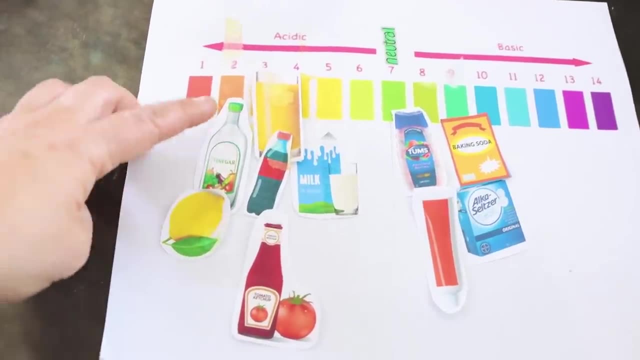 So the baking soda is the basic Uh-huh And the vinegar is the super-duper acidic Good. So it's kind of the same as the lemon. so do you think that if we replace the vinegar with lemon juice, will it still work? 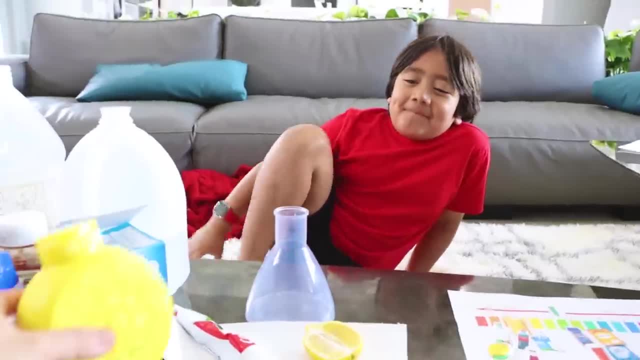 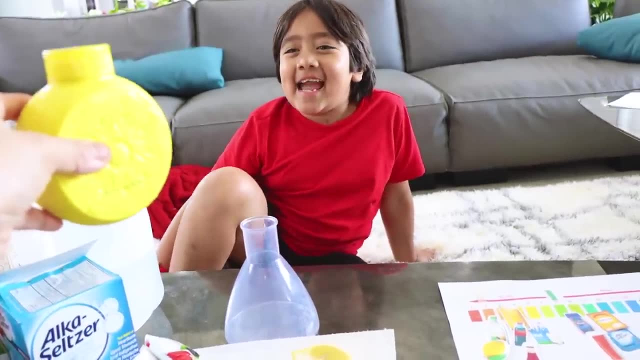 Hmm, probably. Okay, let's find out. Instead of vinegar, we will use lemon juice. Lemon juice, Because it will take too long for us to squeeze, and we're gonna use the one that they already squeezed for us. Yeah.